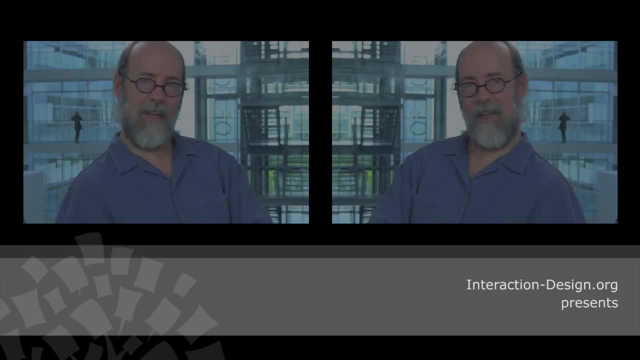 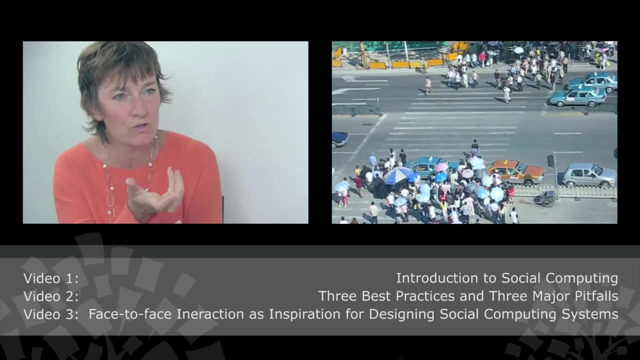 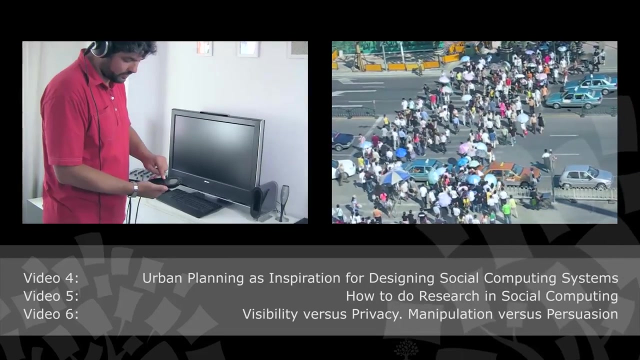 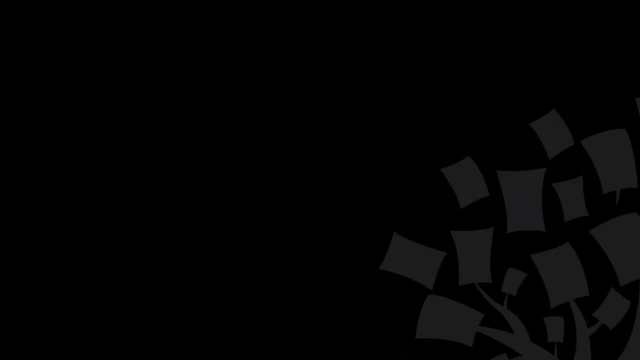 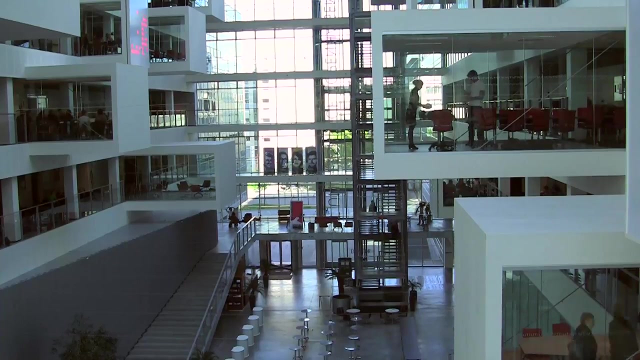 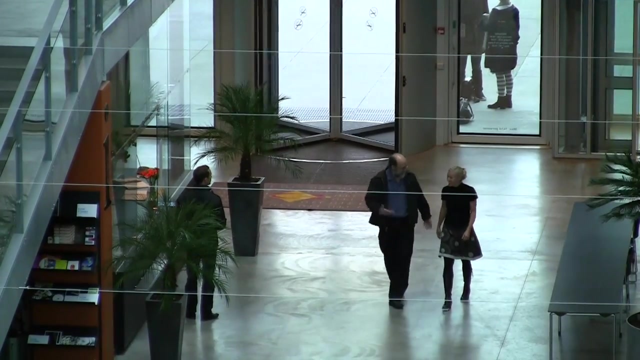 In this interview we're going to meet Tom Erickson. Tom is an interaction designer and researcher and he works for IBM. He works in the social computing group at Watson Lab in New York And he's actually been working there since 97. And before that he worked. 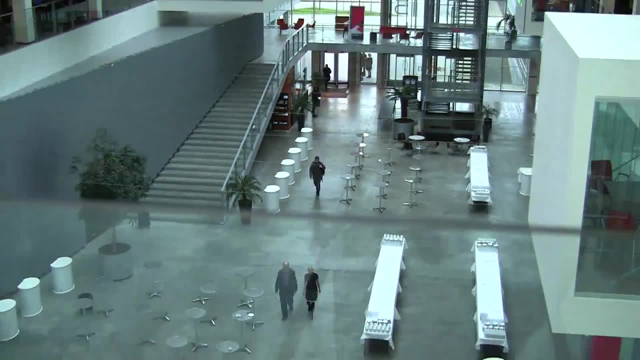 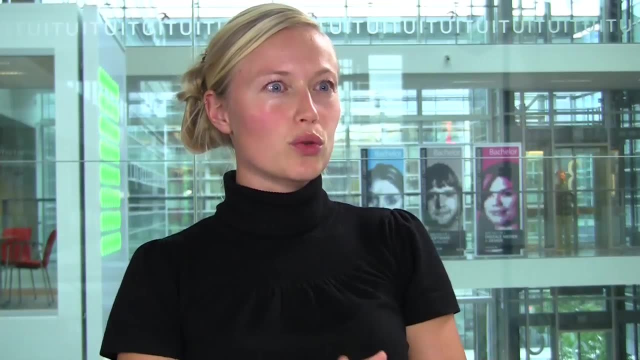 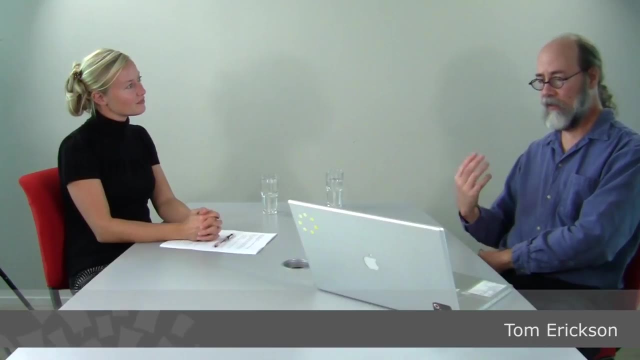 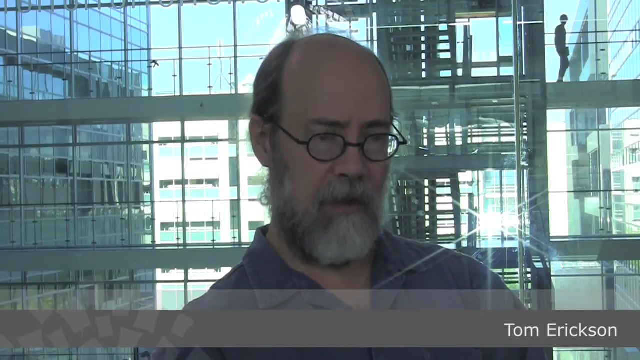 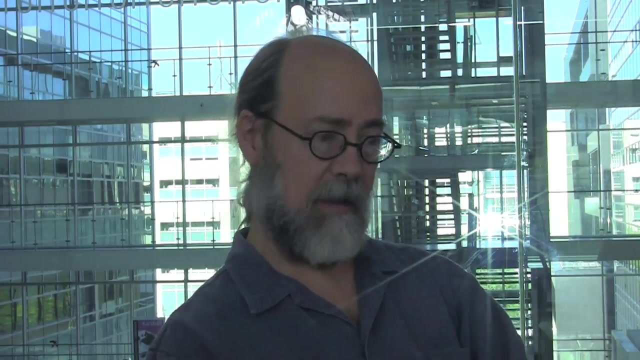 nine years for Apple, So he is an expert on social computing, And this is what we're going to talk about today. So, Tom, what is social computing? Sure, So social computing are systems that support social behavior among people within the system and then make use of that behavior for various purposes, So it can range from: 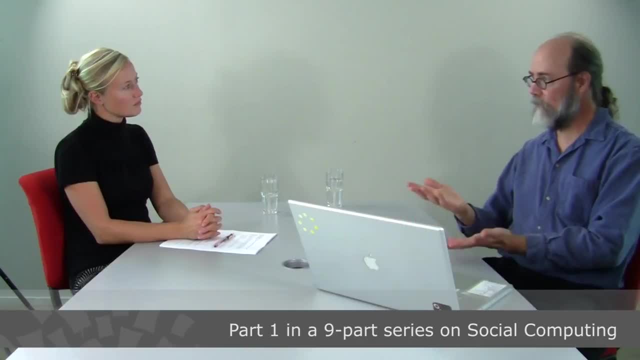 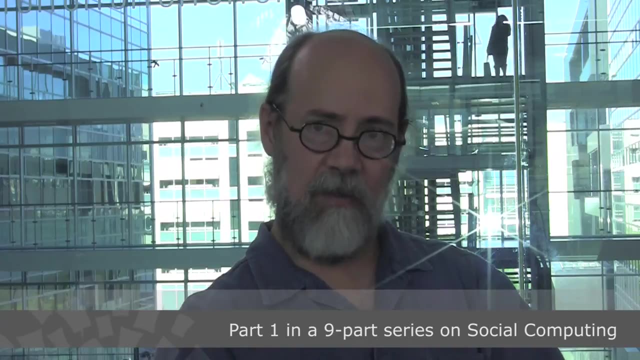 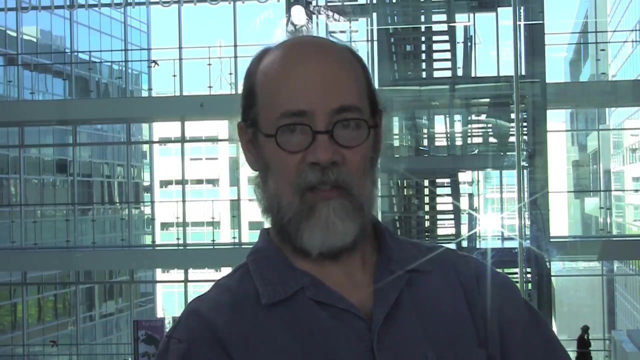 systems that just make use of a few things, So like take Amazon, You go to Amazon and they have people write reviews of books, And then other people come along and as they read them, they say: I like this or I don't like this, And so there are two levels of 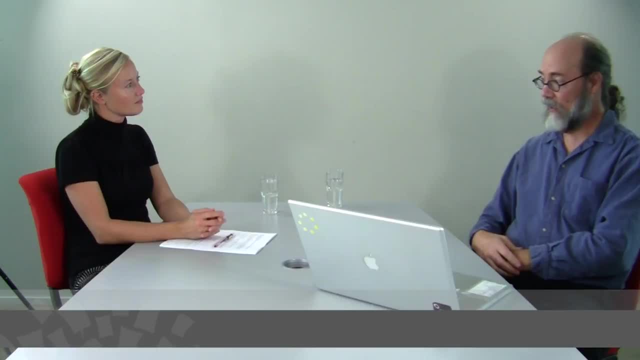 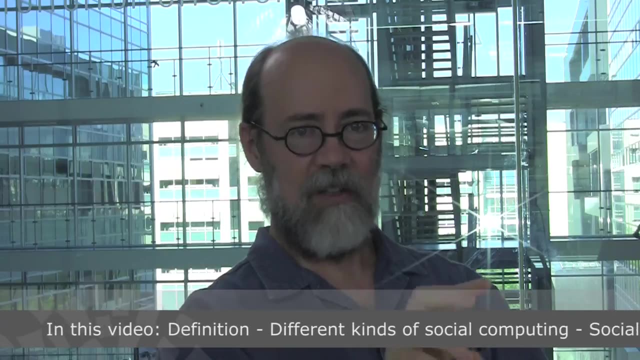 social computing there. One is simply: you can look at a book and you can see how many people liked it and how many people didn't, and read their reviews, And then you can also judge something about the quality of the reviews by seeing how many people thought this was. 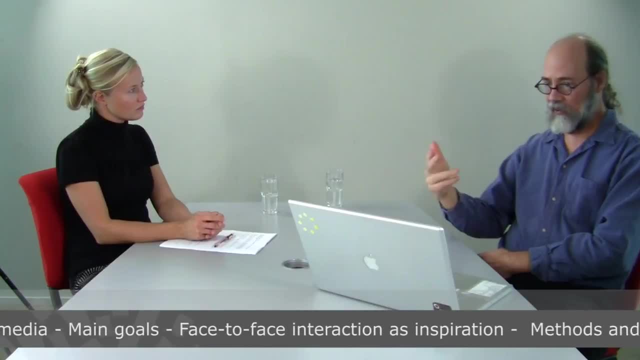 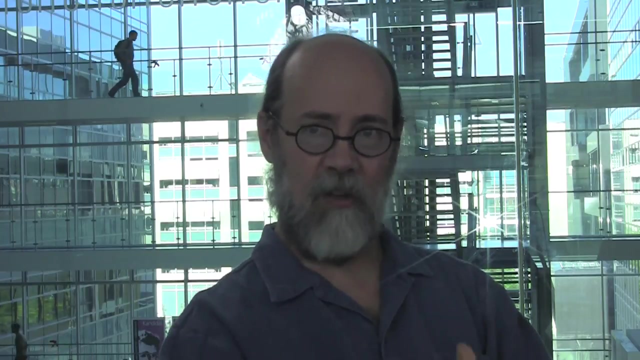 a good review or not, Amazon actually has done something. I think that's quite nice, which is one of the types of reviews they foreground is the most liked critical review. That's a review where they didn't give it a top rating, but a lot of people still found it useful, And I always 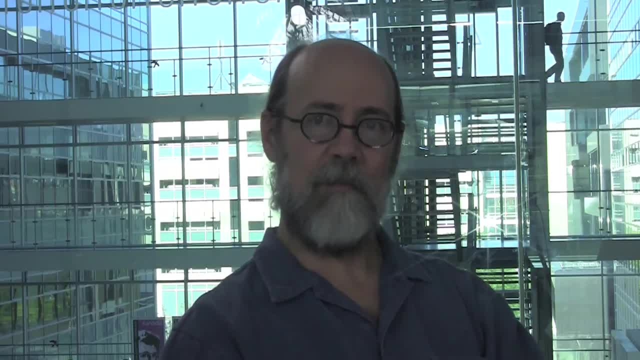 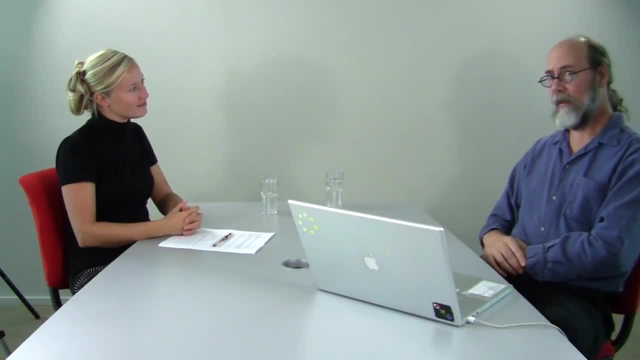 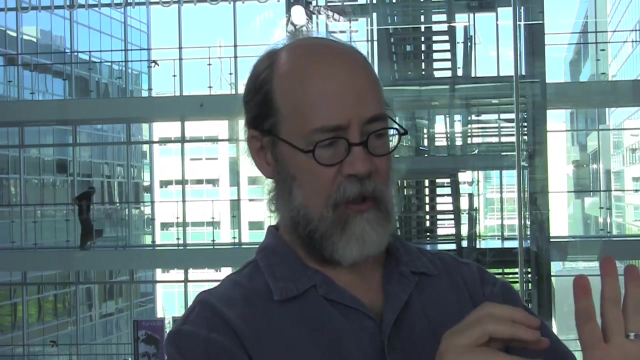 try to go right for that review. Are there different kinds or different types of social computing? Yeah, Okay, Yeah. So there are a couple of answers to that. One has to do with how social computing surfaces in the system. So what I just described- Amazon that uses a few social computing mechanisms. 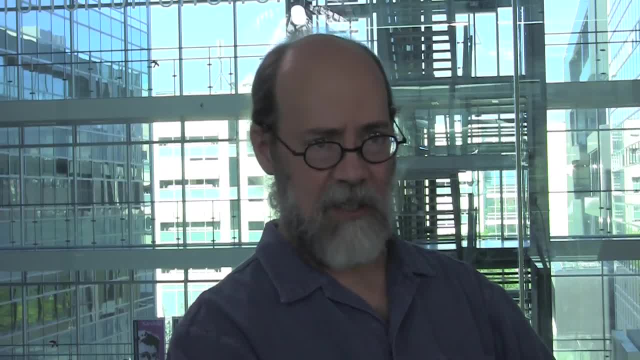 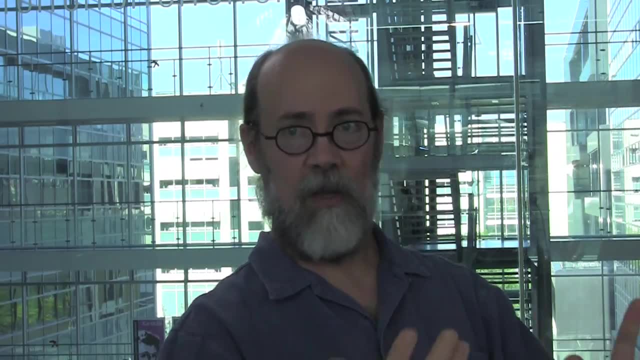 in it. right, You could get rid of the reviews, You could get rid of the liking or disliking ratings, And Amazon would still be pretty much the same. It would be a place to go and buy books or other things, Yeah. 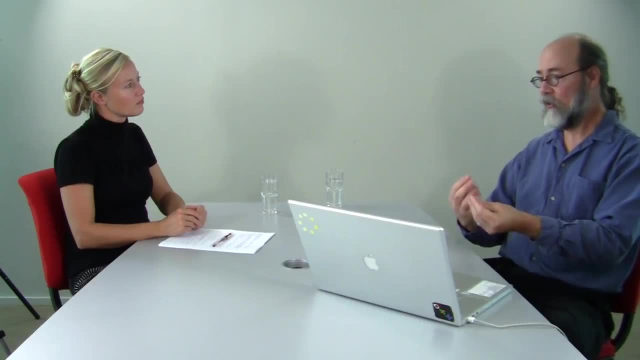 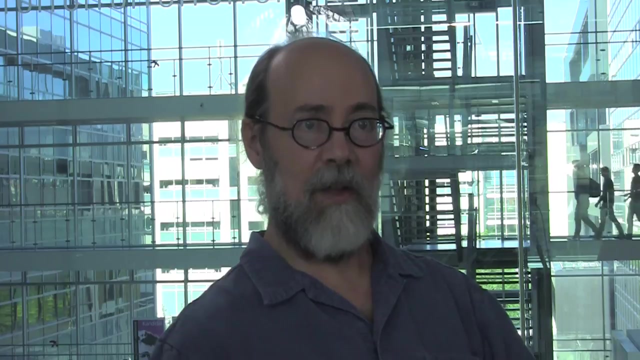 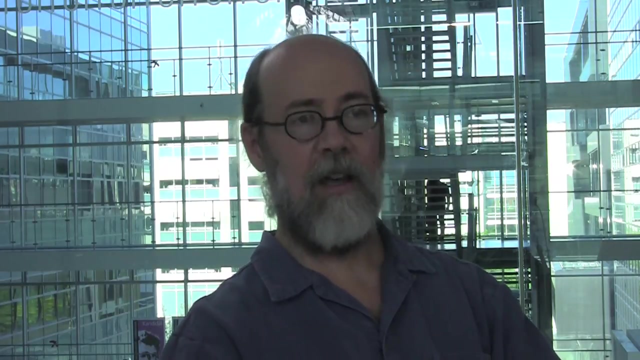 But other types of systems don't just use social computing mechanisms, but they're fundamentally social computing things. So take something like: the canonical example is Wikipedia, where it's all produced by the contributors. So they produce the content, they edit it, they assess quality, so on and so forth. So that's the way it works. 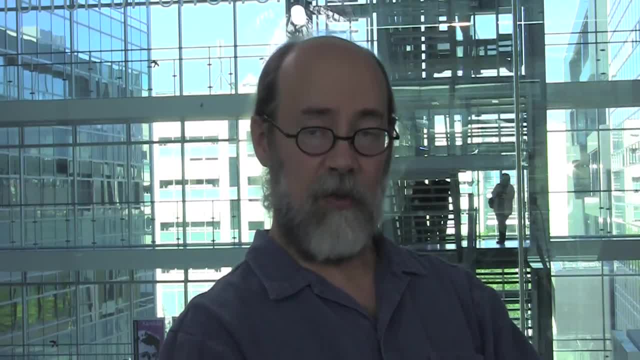 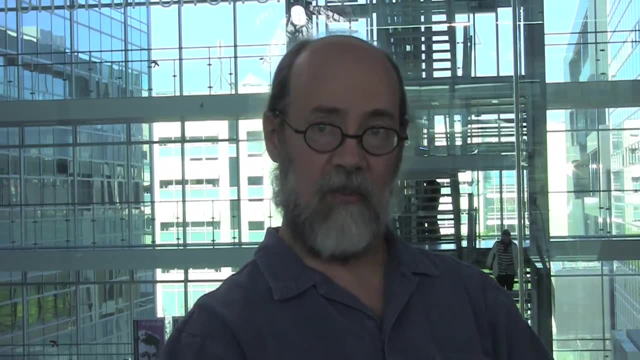 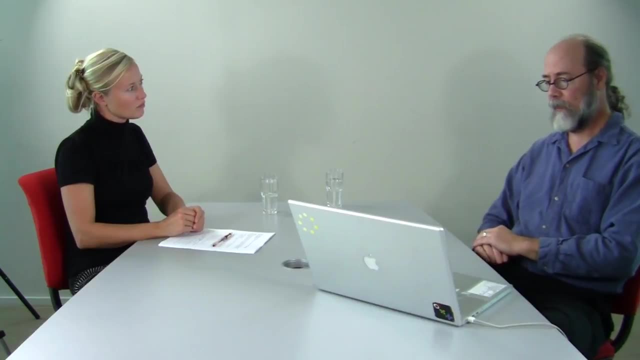 Yeah, Yeah. So that's sort of almost pure social computing, in that it's all coming through users and it's all shaped by social interaction among users. Another way to distinguish between types of social computing systems is that this is something I've been puzzling over. 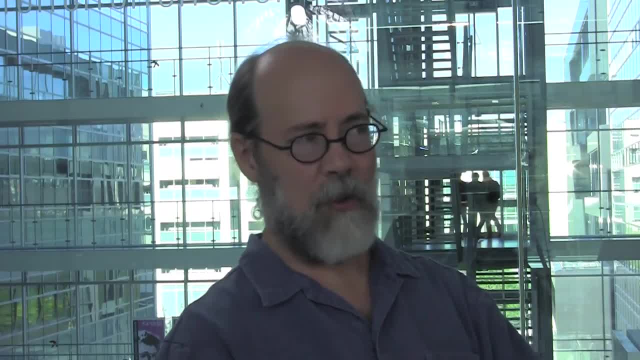 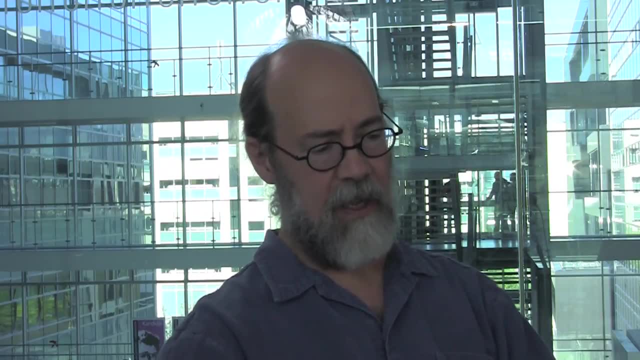 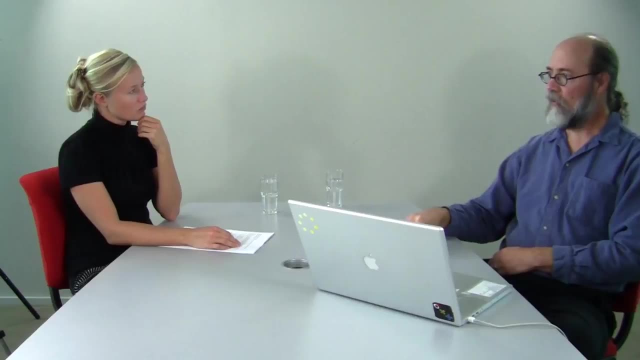 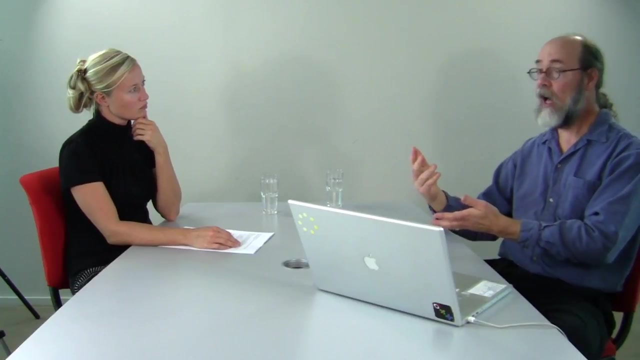 I mostly like examples and I tend to avoid defining things formally, But one of the continuums that you can look at social computing systems along has to do with the type of interactions that are happening in them. So in Wikipedia, for example, the content that is being produced. 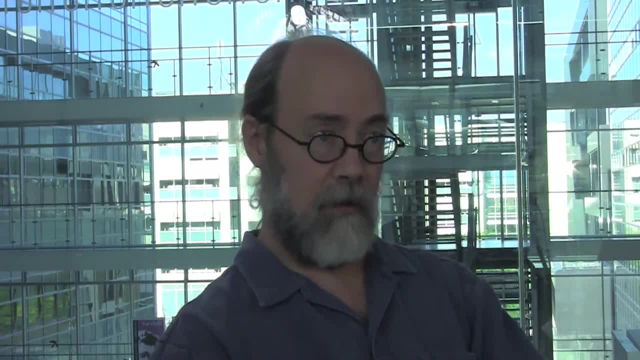 or the knowledge that's being produced, or the wisdom of the crowd, if you like to think of it that way- is coming through the user. Yeah, Yeah, Yeah, Yeah, Yeah, Yeah. So that's something that is very-through conversational interaction, right, Let's. 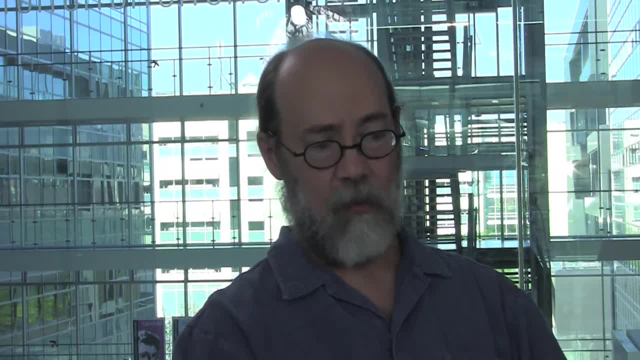 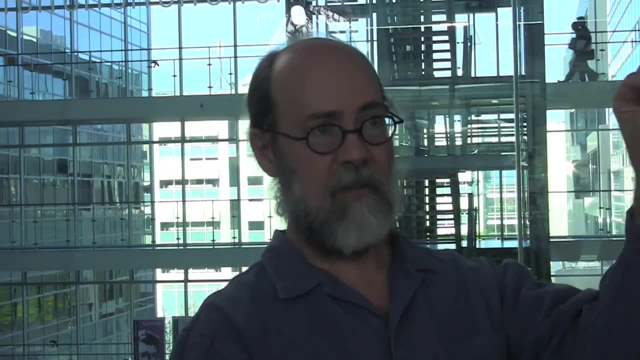 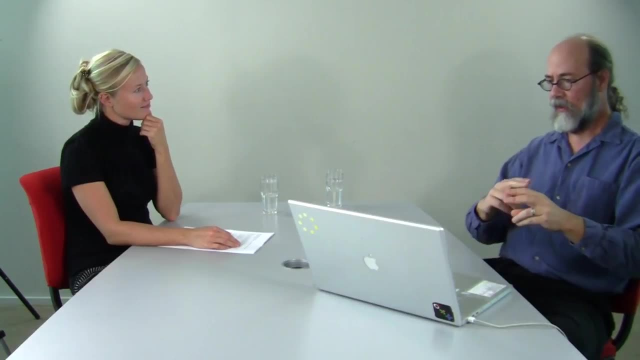 contrast that with another type of social computing system. One example I'm very fond of is that of an online auction. So there you have something for sale, You have an audience of people who want it, And the way in-what people do is they go in and they place a bid. 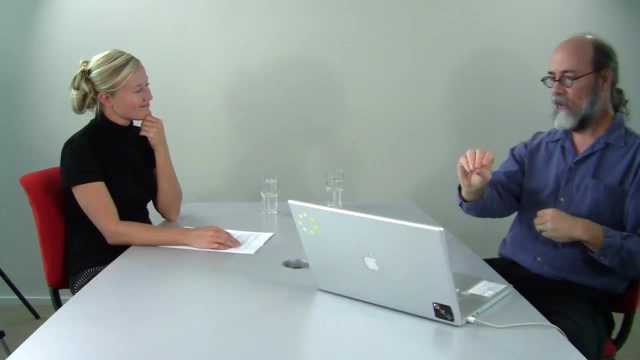 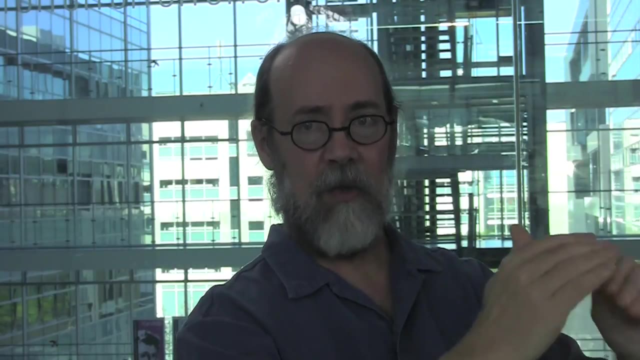 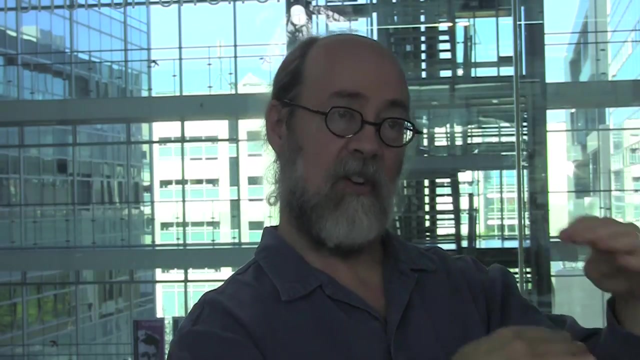 Yeah, You know, I bid for something and then you see that somebody has bid so much for it and you want it more, so you bid a bit more, And so there the interaction is very simple, right? You're simply placing a bid of a certain value and those repeated interactions are, in a sense, 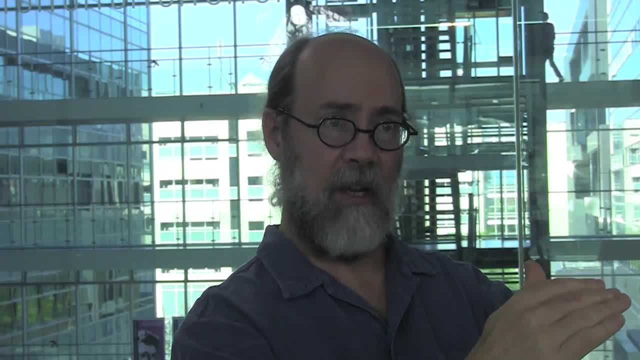 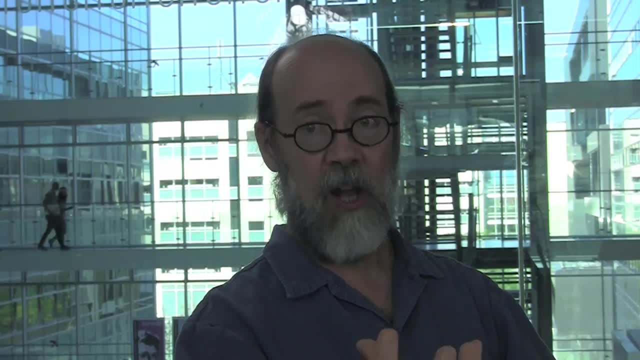 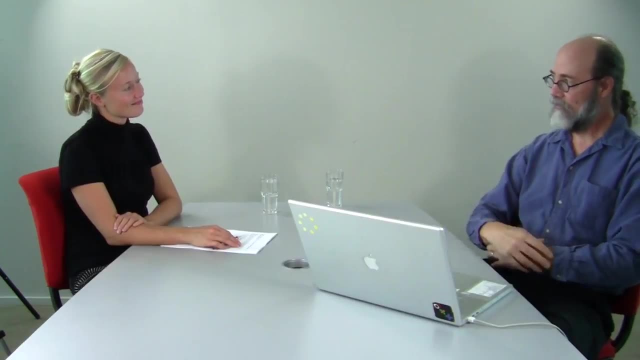 a way of socially computing a price for something right, And auctions are very useful things. so if you have a rare piece of art, how do you figure out what that costs? right, And the answer is: you let people socially figure it out. 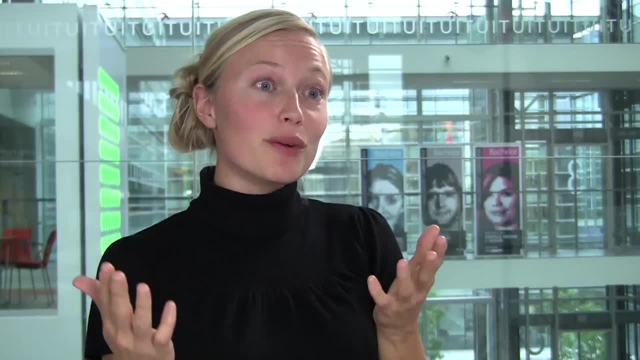 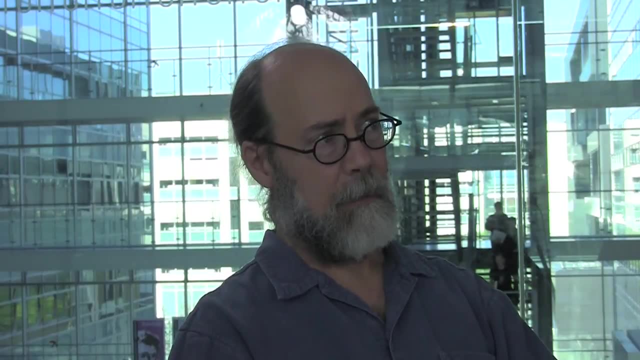 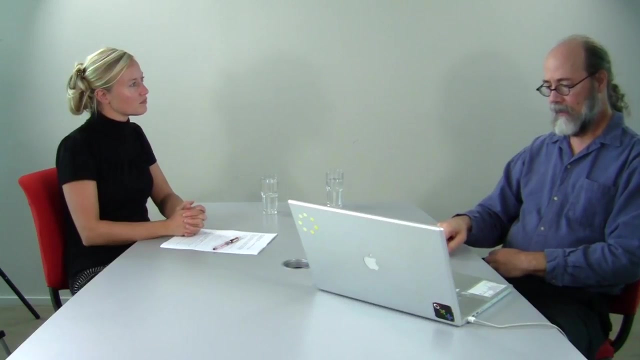 We often hear the term social media. Can you tell us, in your opinion, what is the difference between social media and social computing? That's a hard one. I see social computing as a very general term. I mean, the way I think about social computing is: I think, think of. 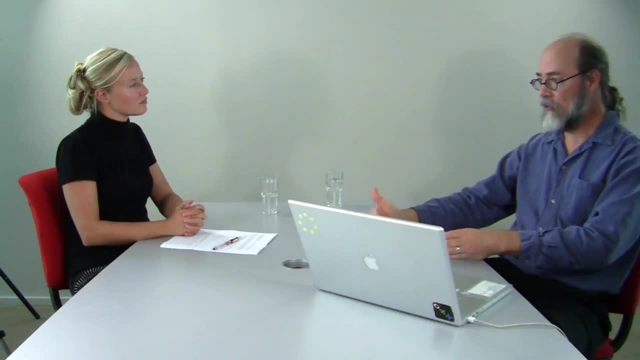 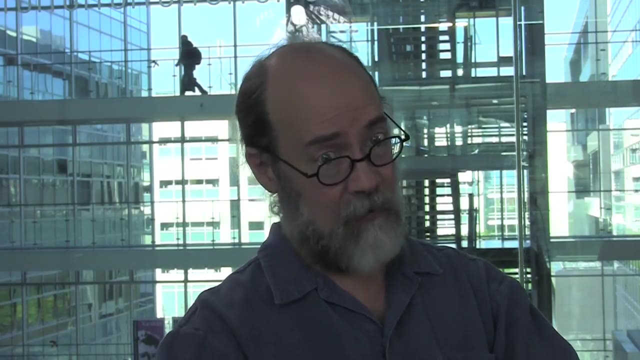 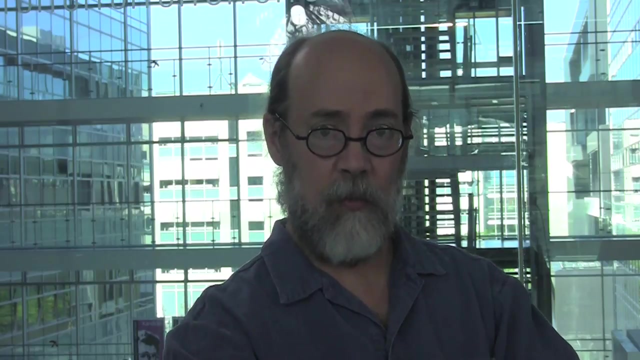 groups of people who are actually collectively computing something, Where I mean computing fairly broadly. it might be figuring out the price for something, like you do in the auction. it might be composing an encyclopedia article, as you do in Wikipedia, but in some sense at a very general level, that's all a computation right. 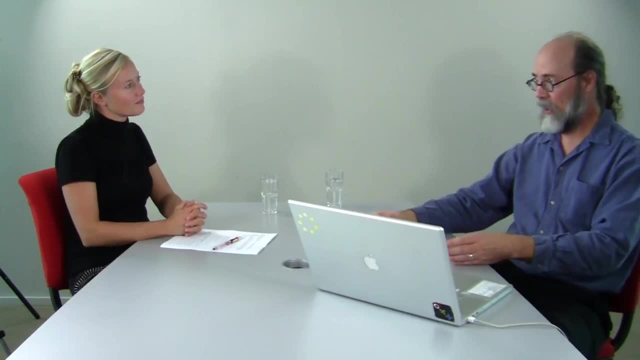 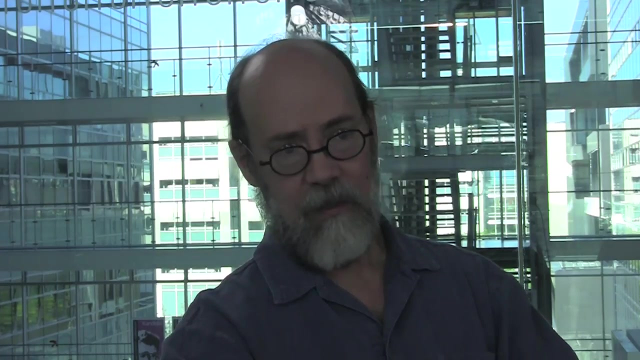 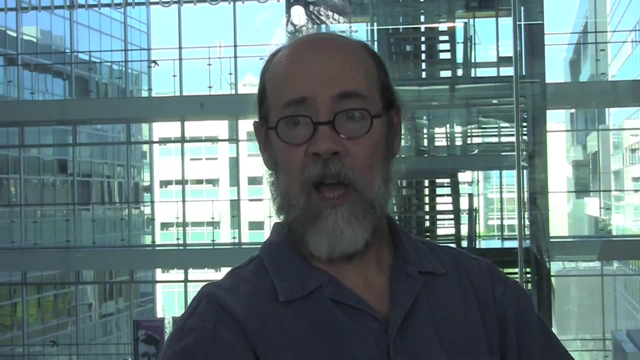 Or a market, is another type of computation. We all collectively place bids for things, and that shapes the price of commodities or whatever it is you're buying and selling. So computing, I think, covers a large range of territory. where So in a market, we're anonymous to one another right? 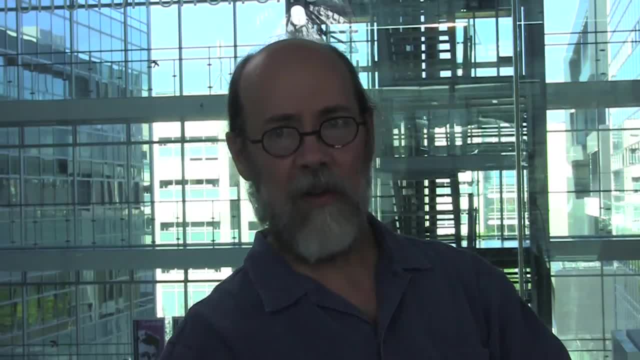 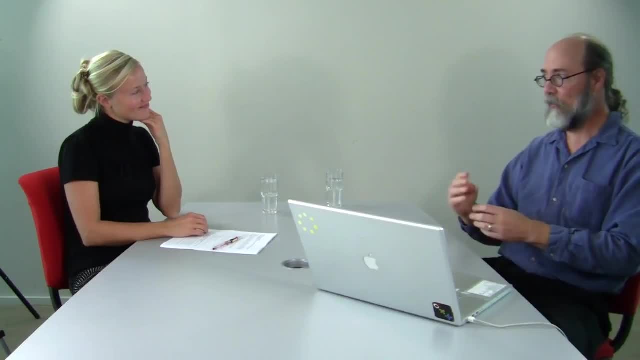 And that's actually important, because we don't want people conspiring to fix the market or we don't. they don't want us conspiring to. you know all bid. I think they call them shills in auction, where you insert people who were false bidders to sort of drive the price up. 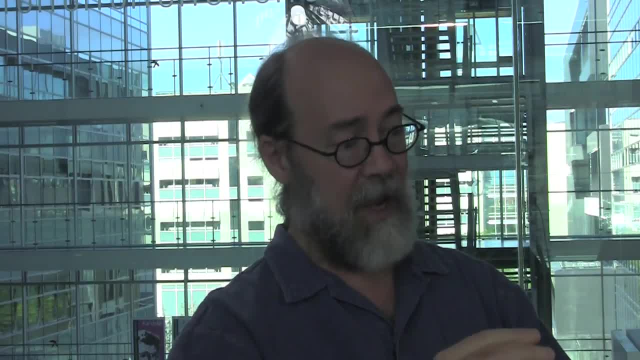 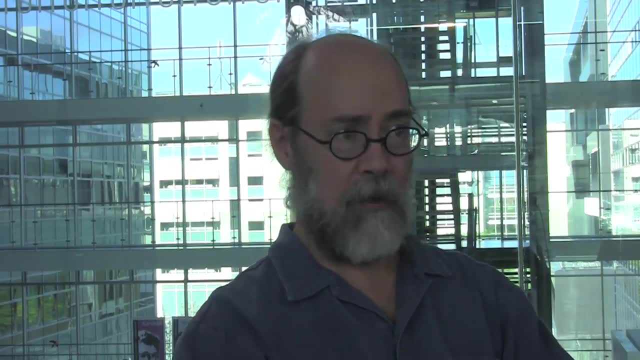 right. So in social computing systems you might have cases where people are interacting a lot, very deeply, getting to know one another, like in Wikipedia, or you might have a very, almost anonymous type of interaction where all I know about you is that you've just outbid me and how. 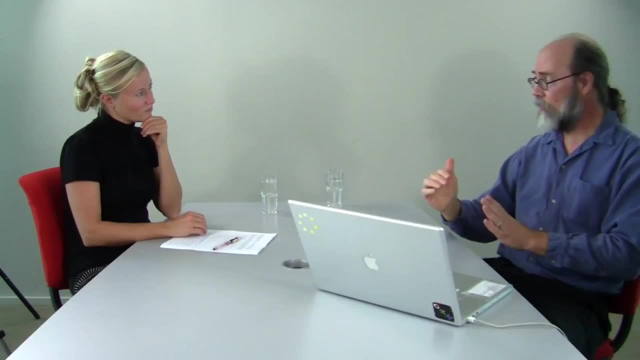 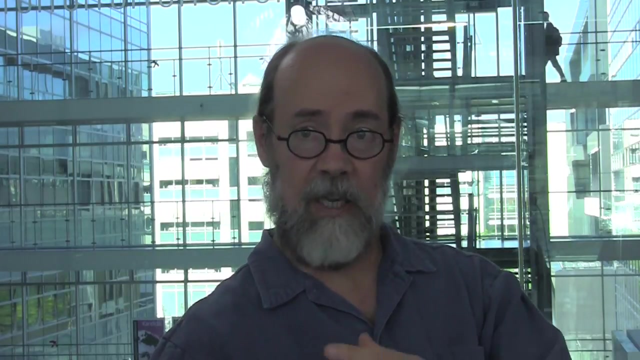 am I going to react to that? So I think social media- the way I think of the term- has to do with people actually having a rich communication among them, right? So Wikipedia, it's not all social media but, for example, the talk pages are clearly social. 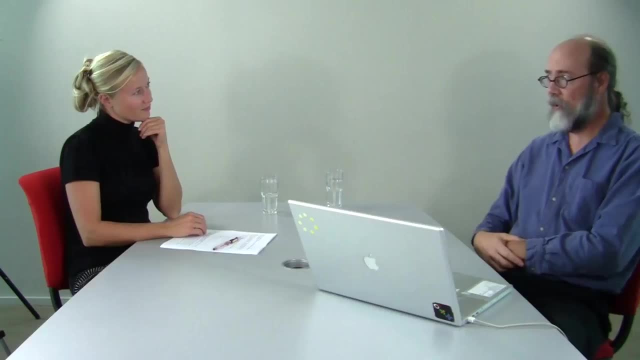 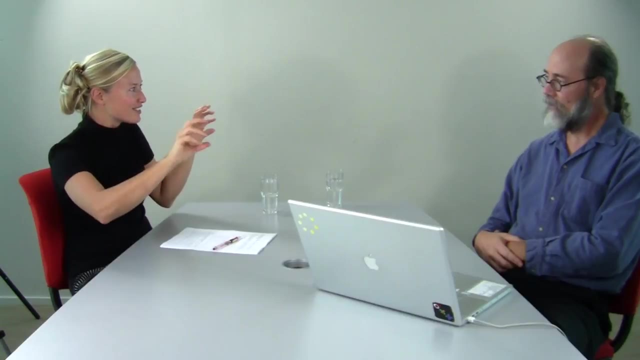 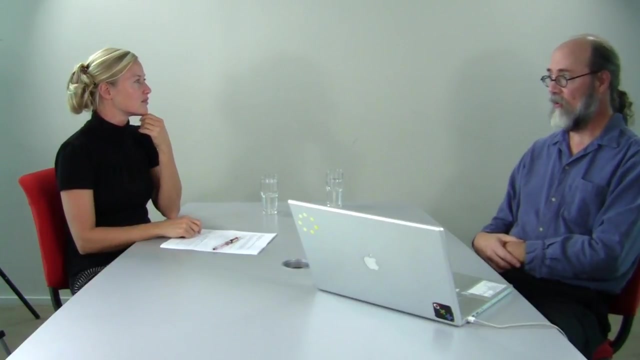 media, whereas an eBay auction I wouldn't call that social media. Okay, So it's actually a scale and you can say it's more or less social. Yes, yes, Yeah, You know, and you can imagine that. you know, you could take an online auction system. I. 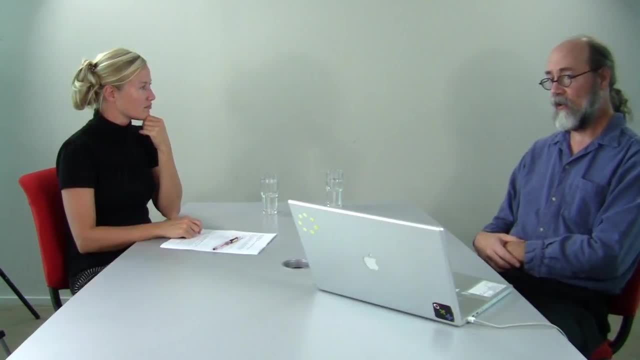 don't know to what extent eBay does this- I haven't looked at it in a while- but you can, you know, imagine creating some kind of online community of customers who are, say, interested in you know some type of art that they collect through eBay. 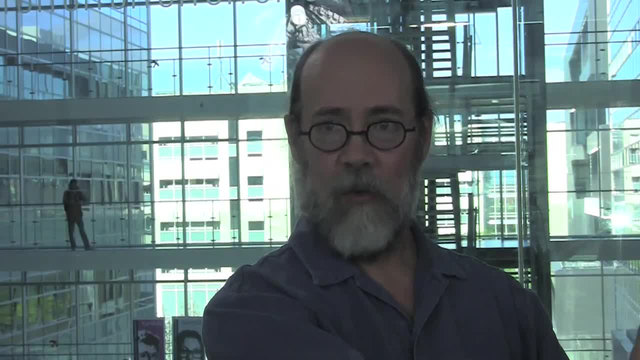 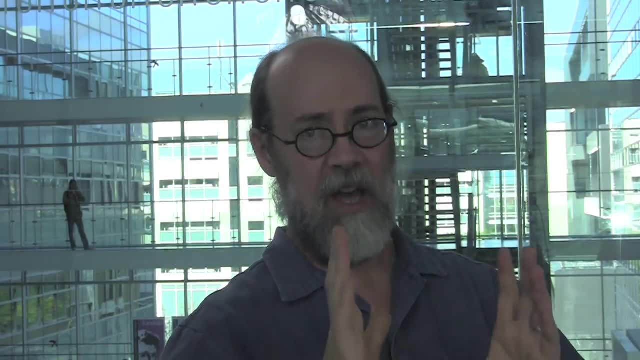 And so you might have a little place where there's, you know, very rich social interaction. that would be social media. but then you have other niches, the auction, where people go in and they're anonymous and all you do is bid right. 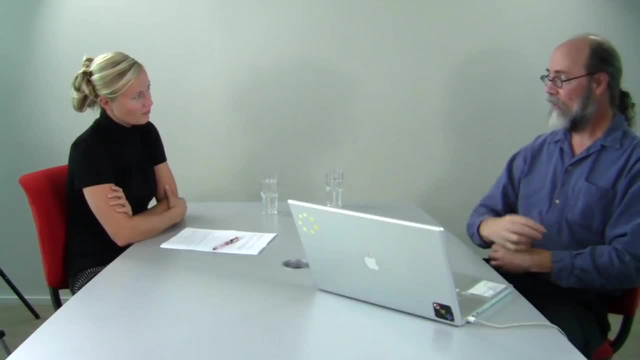 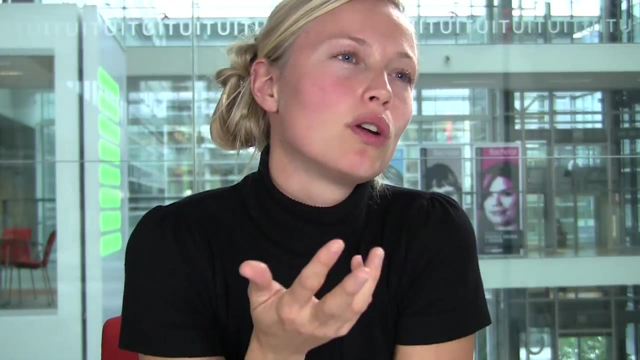 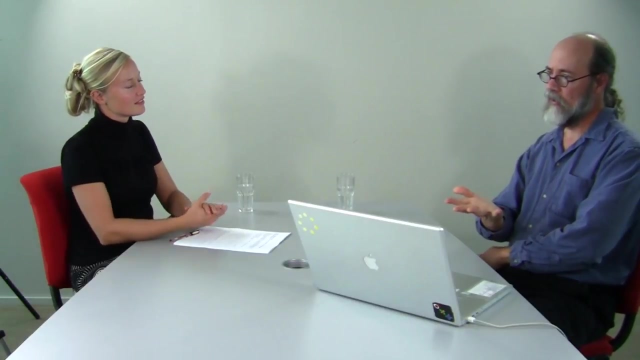 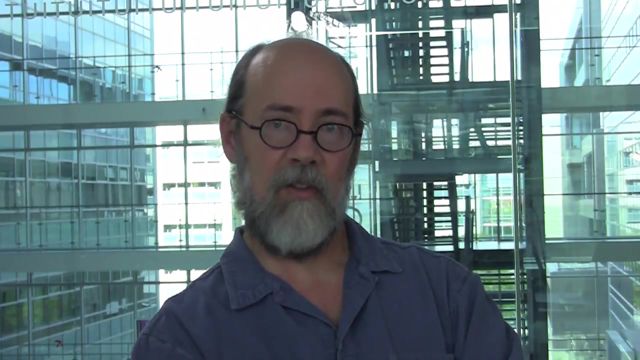 So you can compose all these different things together, depending on the type of interaction you want to support. Yeah, Can you pick out one main goal of social computing? Well, for me, the main goal is interaction. Yeah, In face-to-face situations, at least in the ones that work well, they're interesting. 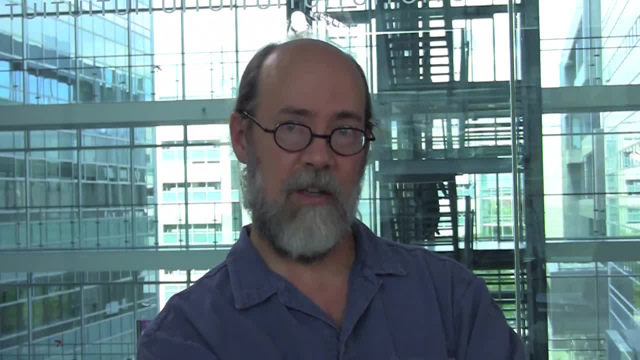 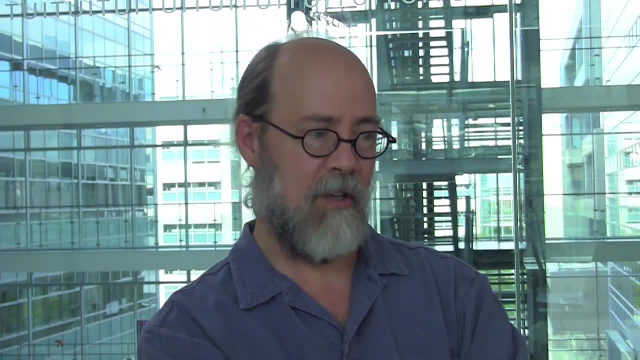 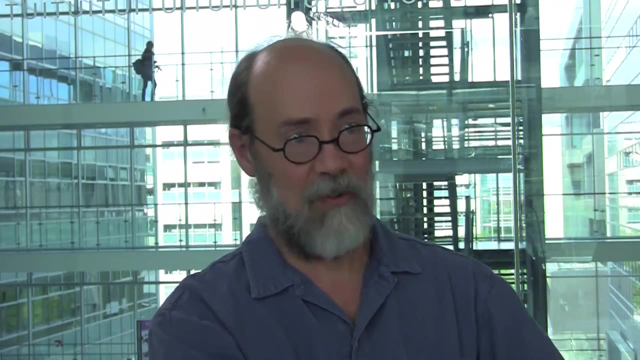 they have a life to them, they give a bit of energy, they have some spontaneity. To me they're, you know, a good face-to-face situation, where you're with people and things are happening is just energizing and alive. and you know it's, I think, something that's. 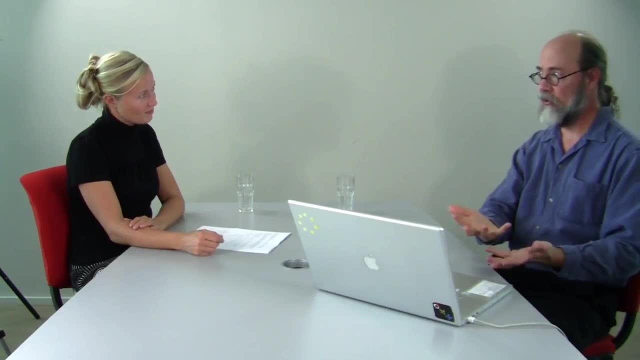 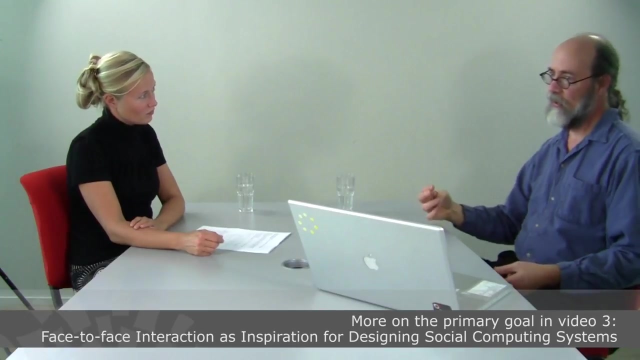 very fundamentally human right At the base. we're social creatures and we get something from that interaction, And so I guess, when I think of the sort of primary goal for social computing, it's to create online places or applications or even services, call them what you may- that 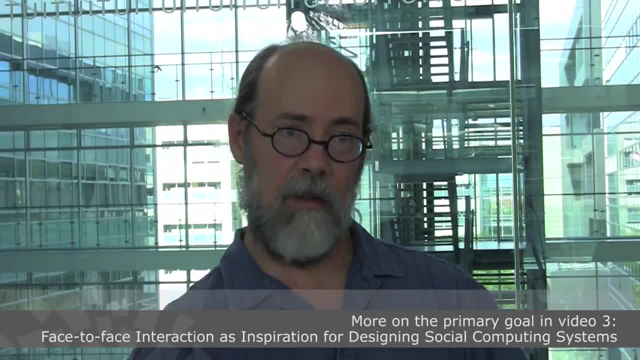 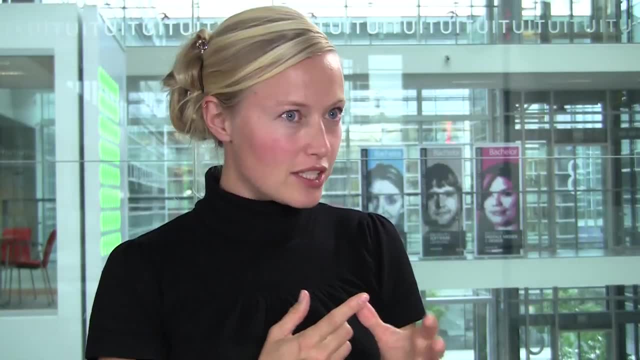 have some of that life to them that you know is fundamental to being human. Can you give us some examples of some of the main goals for social computing? Yeah, Yeah, What are some of the methods and theories you use to approach this goal? 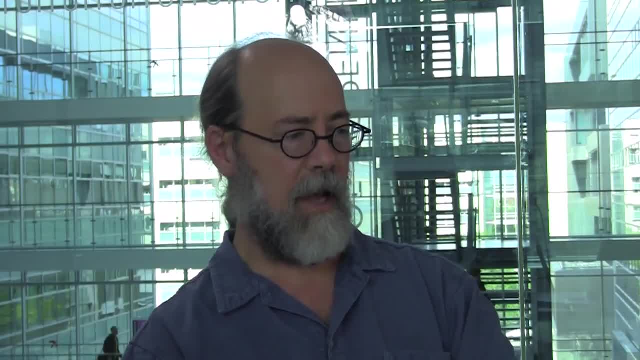 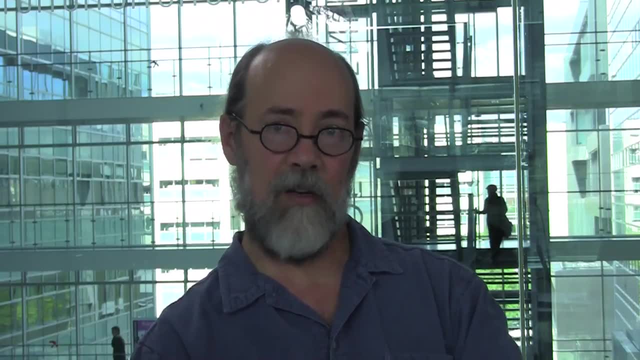 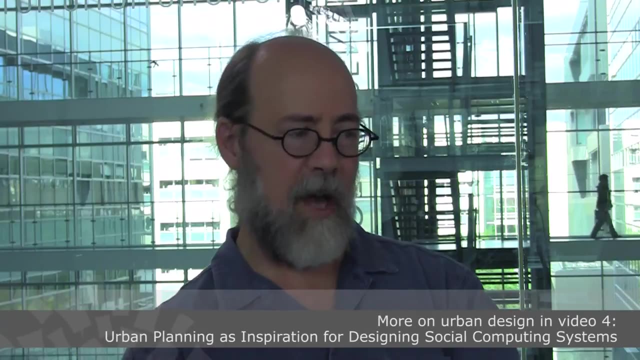 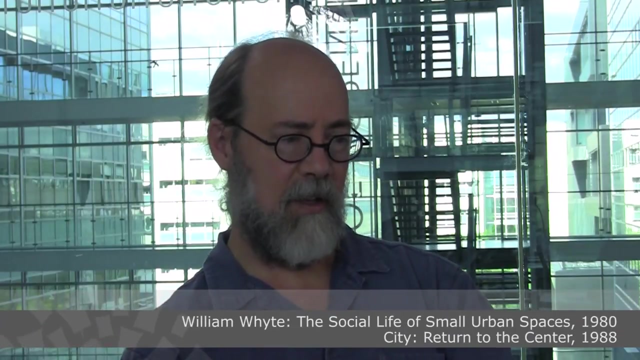 Let's start with the theory. I draw on a couple areas of theory. One is actually for a couple of decades: I've been very interested in urban design, and then also there's a body of anthropology that studies behavior in public places. The best, most famous example of this is William White, who wrote a couple of books, one called 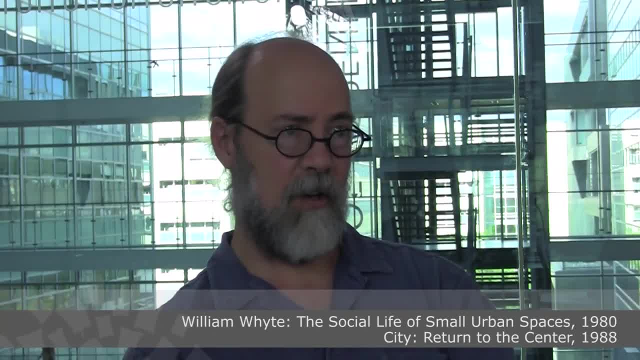 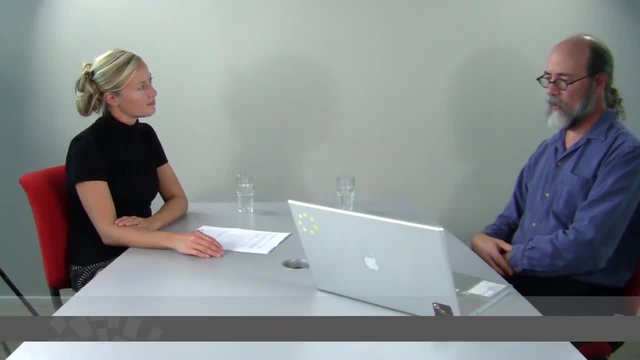 The Social Life of Small Urban Spaces and then a larger book that includes that actually called City. Return to the Center, And White looked very closely at how people interacted in public spaces and he observed a lot of interesting things that I think have direct applicability. 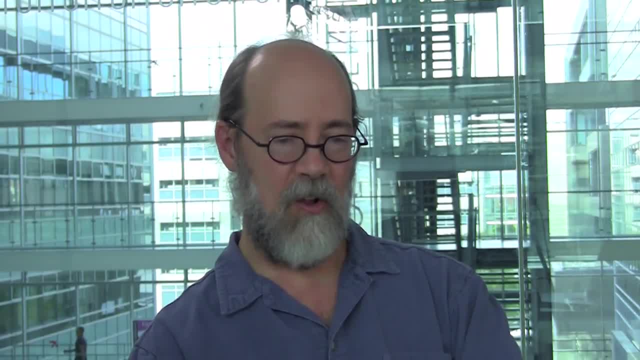 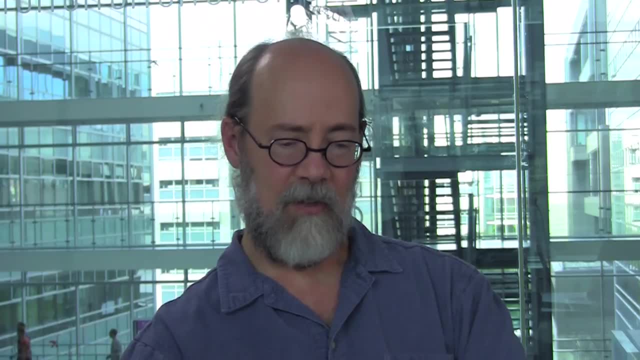 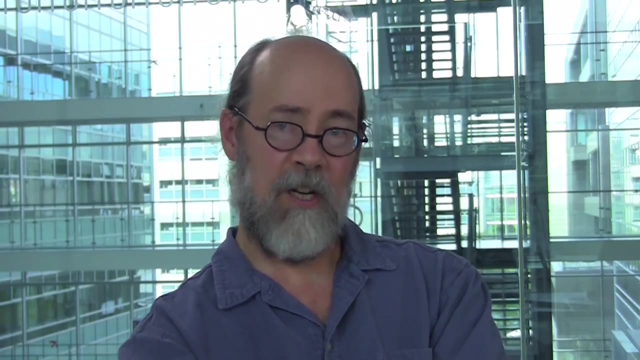 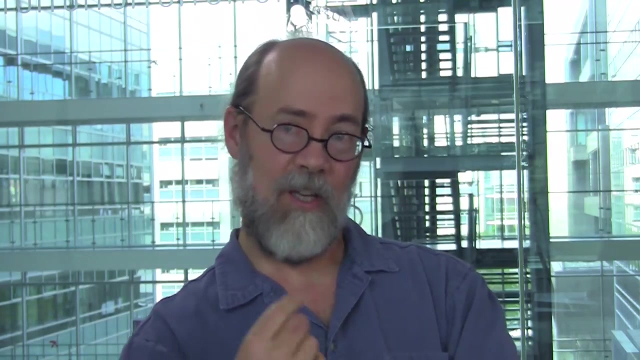 So one thing he talked about he called triangulation, and by triangulation what he meant is something would happen in a public space that would cause two people who didn't know one another to start talking right. So it might be walking down the street and seeing a juggler or somebody walking a new. 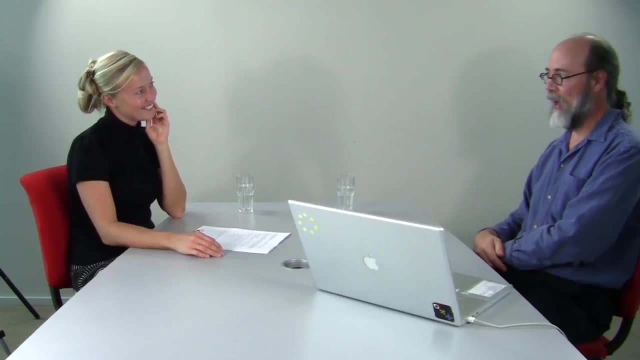 puppy down the street that often gets people to stop and oh, what a nice puppy. and there's a focus for the interaction and there's a reason for people to approach and begin talking. So that's one example of that type of work. 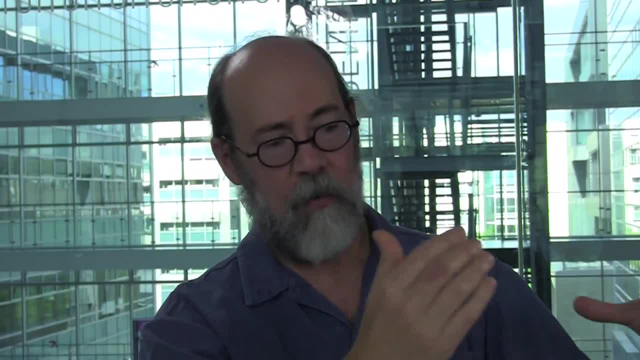 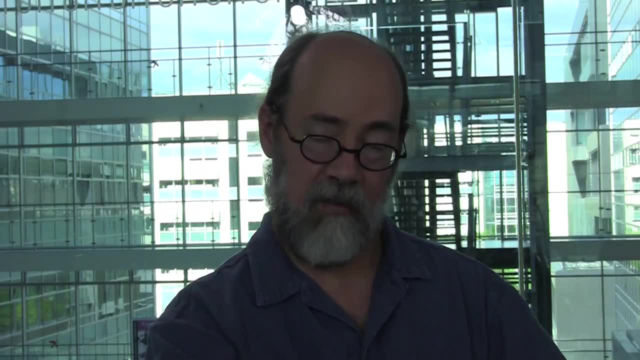 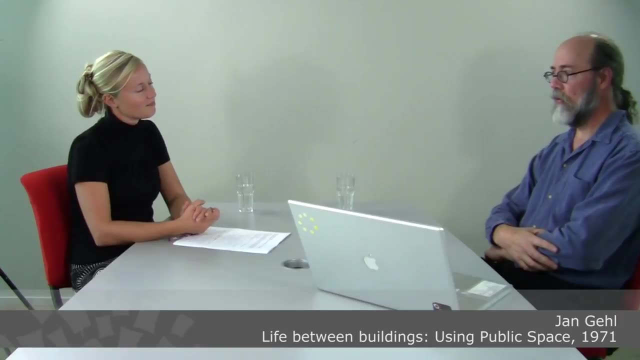 In addition to so there's so urban designers think a lot about how to structure spaces so that they can support that kind of interaction. There's a Danish architect by the name of Jan Gehl who has a book called Life Between Buildings, and he has some very interesting ways of thinking about public space. 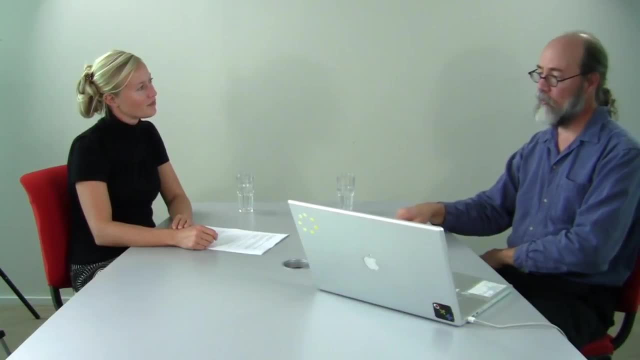 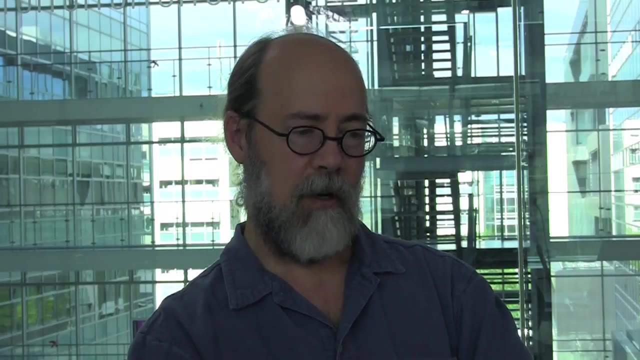 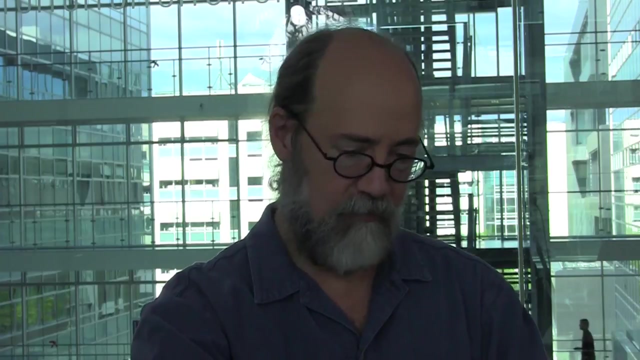 He designed things and he thinks about things in terms of interactive radiuses. So he talks about how far he talks about a radius. He says, Well, if you're within this distance, let's say it's 50 meters. I don't remember what. 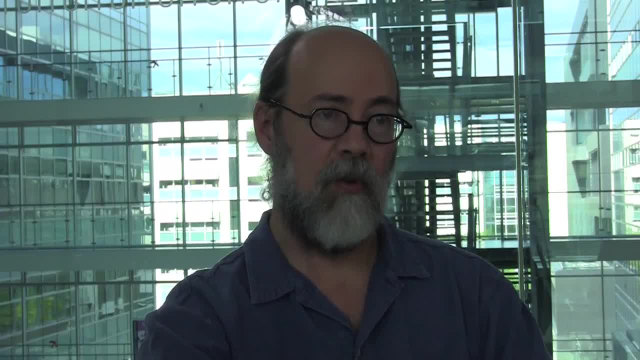 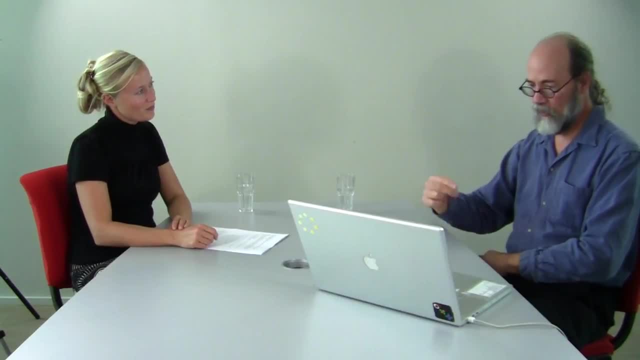 his numbers are, you'll be able to notice somebody that you weren't expecting to see. but you know, If you go into a place looking for somebody whom you expect to know, ah well, you can see them at a longer distance. maybe you know 150 meters, and so he looks at spaces. 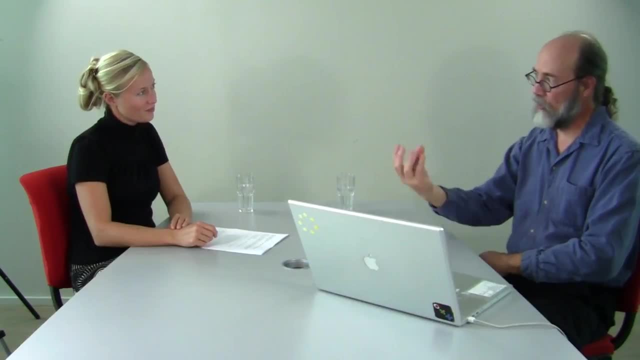 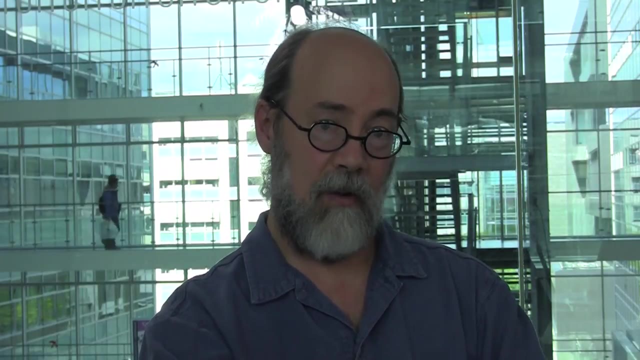 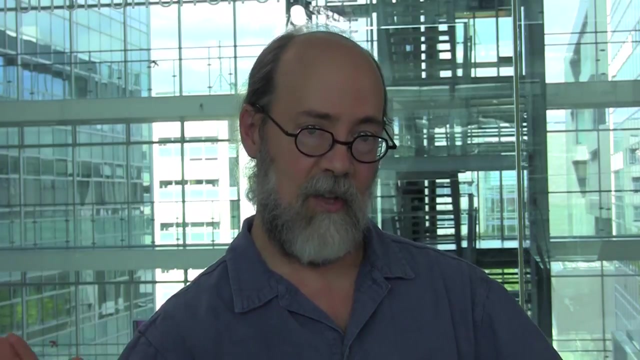 in terms of the types of interactions they might support And how close you would have to be to get that interaction. So that's another interesting way of thinking about designing well, either face-to-face situations or online spaces, which is what you have to provide to make a particular type. 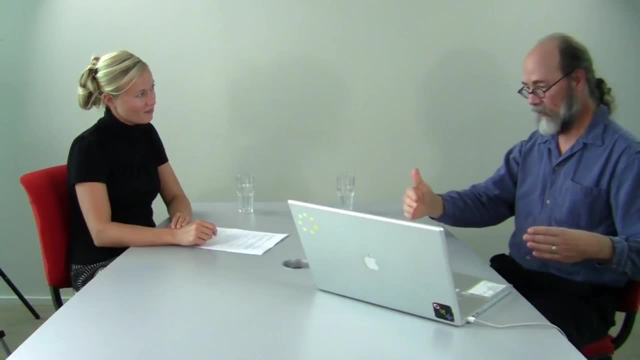 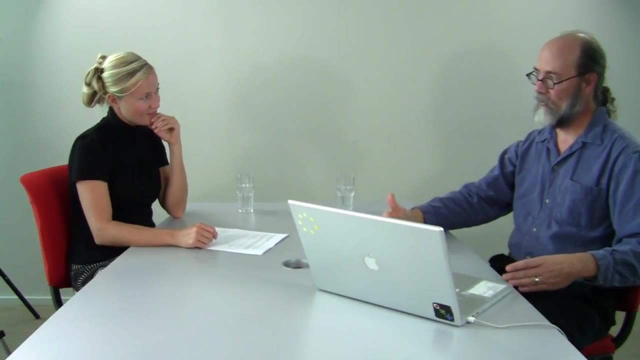 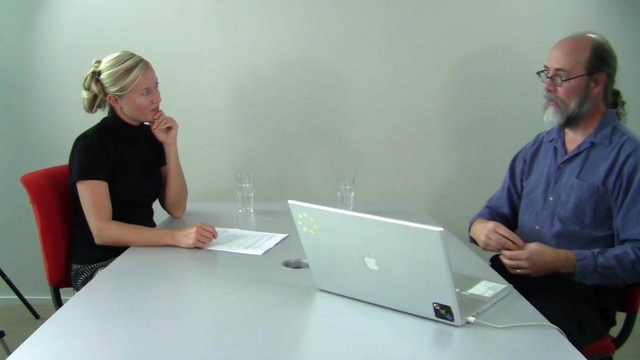 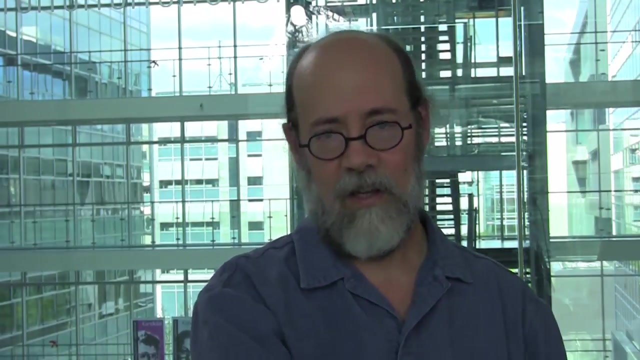 of interaction possible And in urban settings. what you want is you want a space to afford many different types of interactions. right, So A good public square, for example, has places where people can meet one another. right, I'll meet you by the big clock, or I'll meet you by the statue of so-and-so. 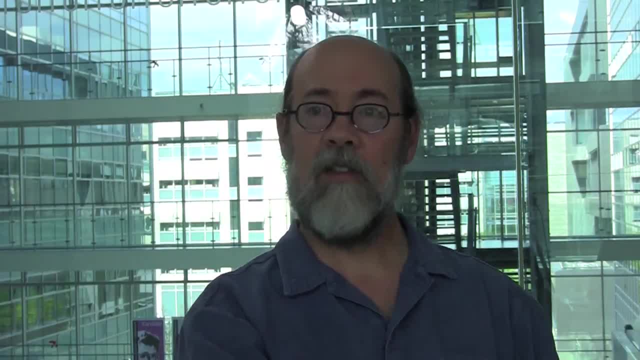 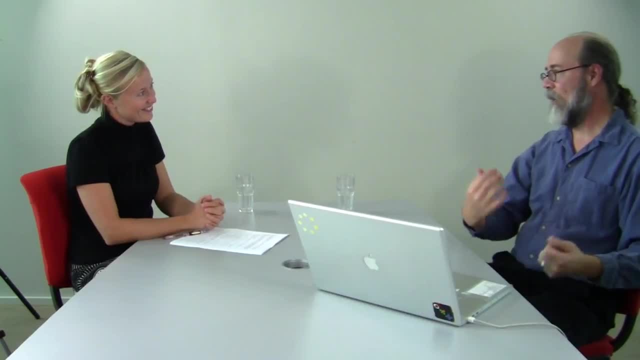 Can you translate that to a social computing system? A very good question. Often you can't, but you might well want to. So certainly there are 3D online environments like Second Life right. So now we could say: let's go into Second Life. 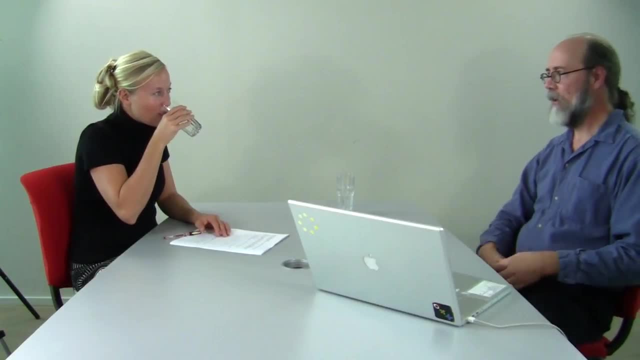 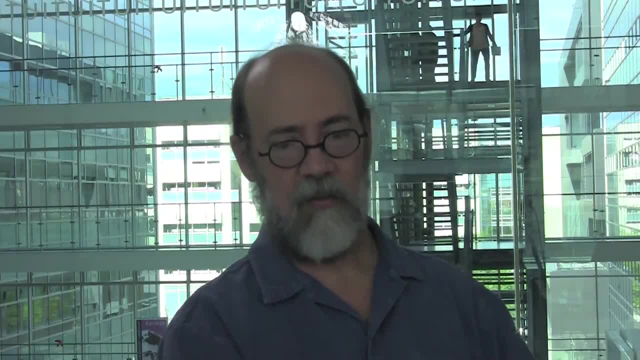 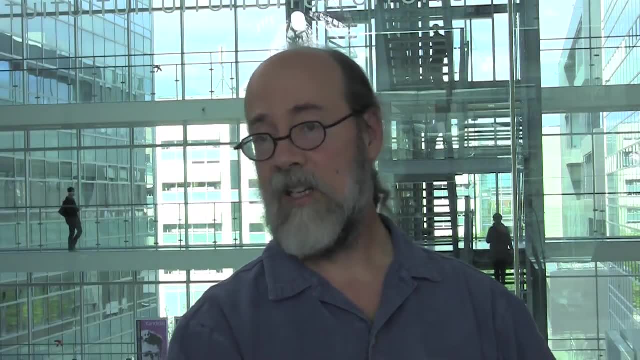 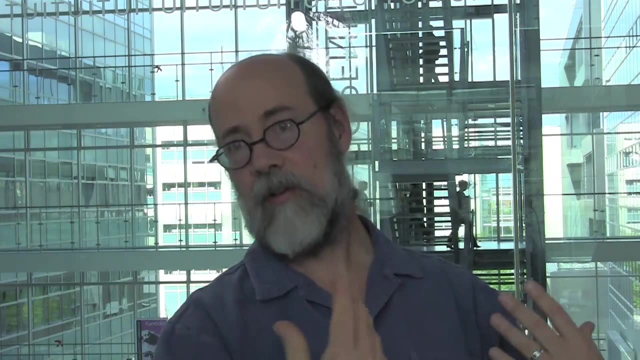 pyramid. So that's one thing. To go further back in history, looking at things like IRC, right, So you could, you could agree to meet somebody in a particular IRC channel at a particular time, So you, you can do that. Or an online community where you have- you know a, you know a, you know a, you know. 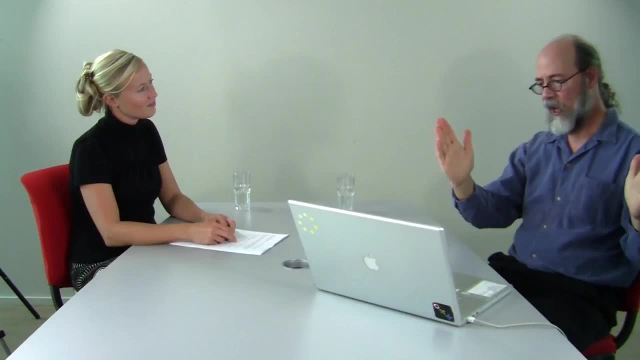 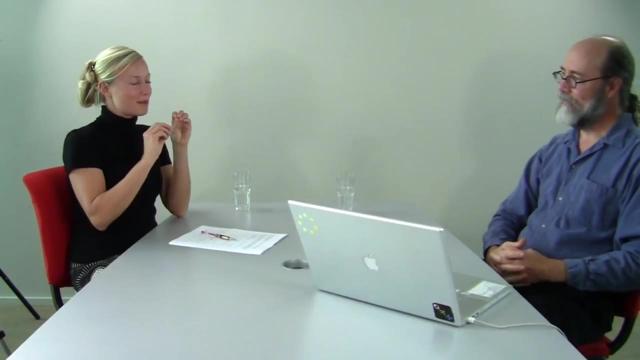 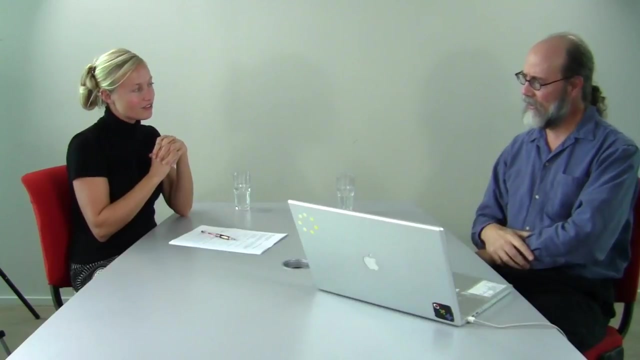 general conferences and within conferences, you have topics, right? oh, let's go and talk in this topic. okay, so if we take a step back, how did research into social computing start? are you, are you asking about the field in general? or yeah, the field in general? well, i would trace it back to. 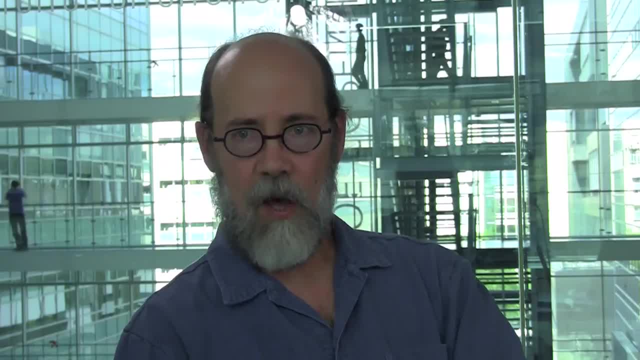 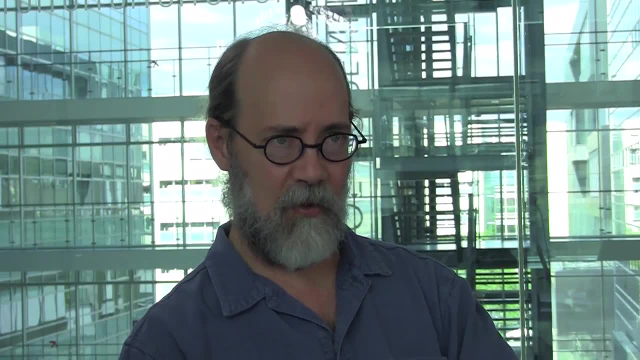 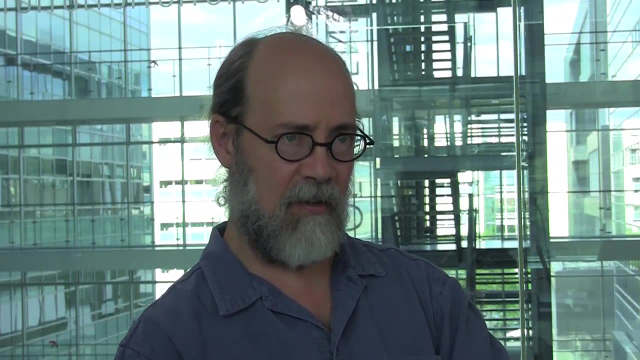 i guess the study of online communities. i mean social competing. you know social computing is a relatively recent term i i don't know exactly when it started, but you know, certainly not uh as as a name that people use commonly before the the late 90s at the earliest uh. but you know social computing in the sense that. 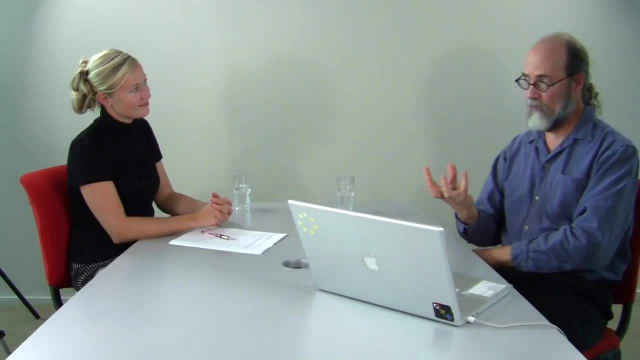 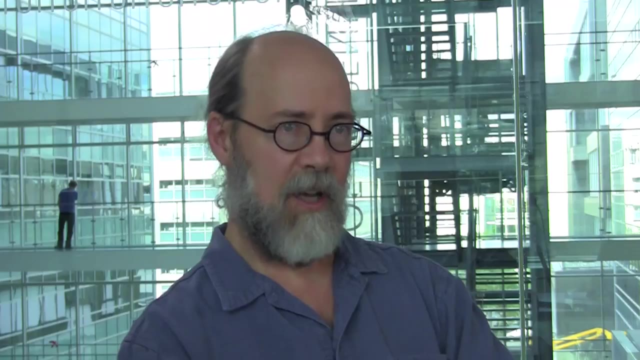 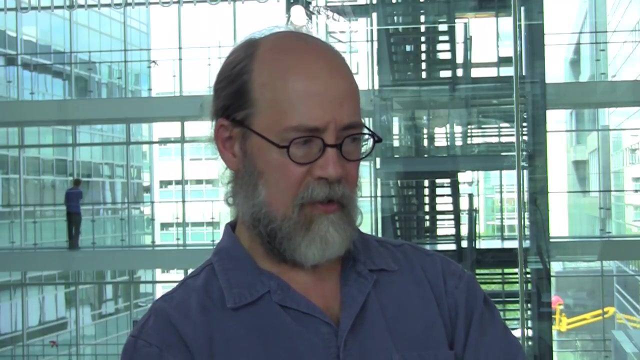 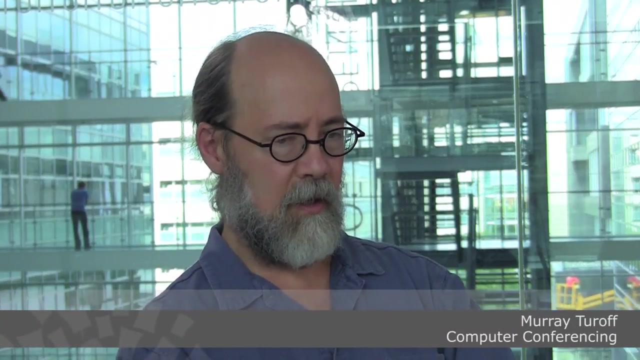 you have systems that are trying to support social behavior among their users and to make that behavior either produce useful things or make it useful on its own. that certainly goes goes with the way back to online communities. i think uh, uh, the the earliest uh online community- back then they called it computer conferencing- was uh. 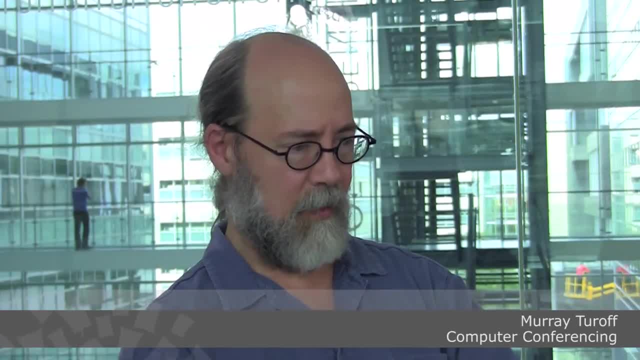 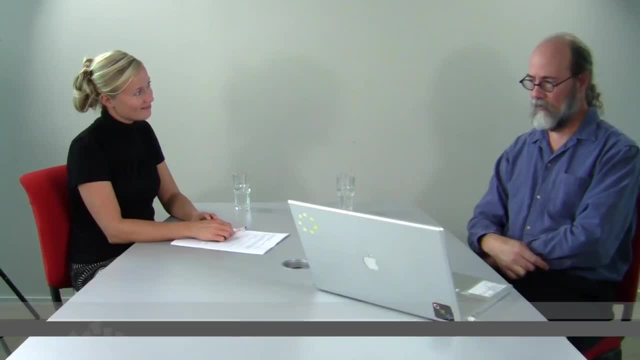 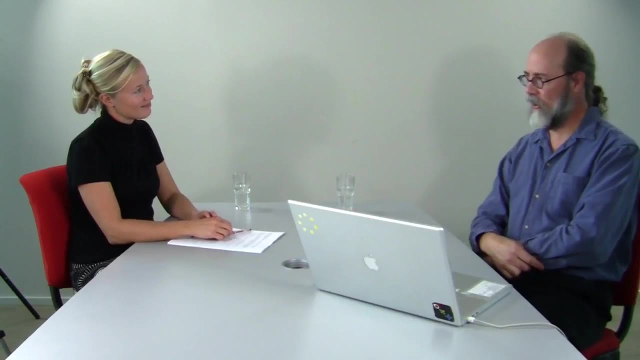 murray turoff's system used in the us in the seventies and that was a private system actually used to administer the us wage and price control freeze of the nixon era. uh, so that that probably was not social computing. that was just a bunch of. 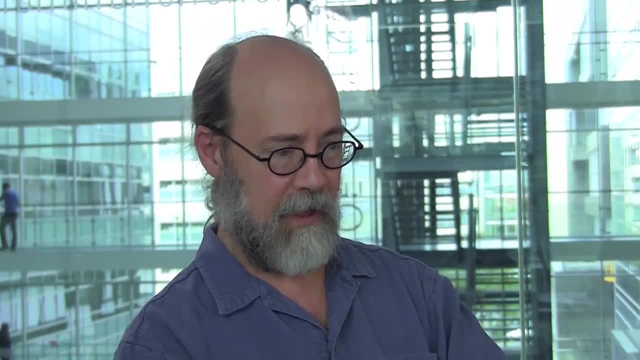 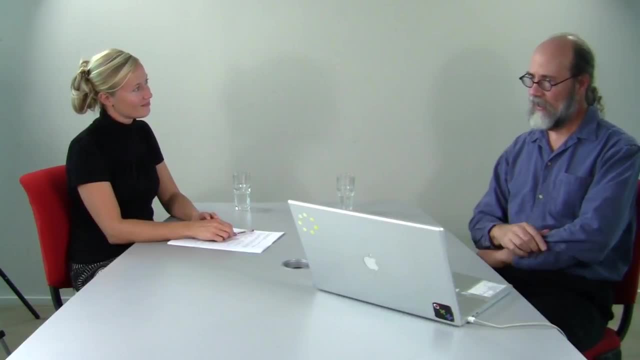 uh, policy. uh, people trying to sort of regulate things. but not long after that, you saw the emergence of of more public online communities. uh, i don't think i can pull the history out in my head, but uh, there were some early chat communities. uh, turoff went on and built a system. 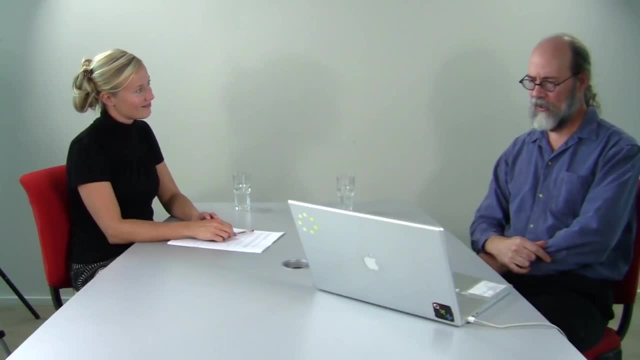 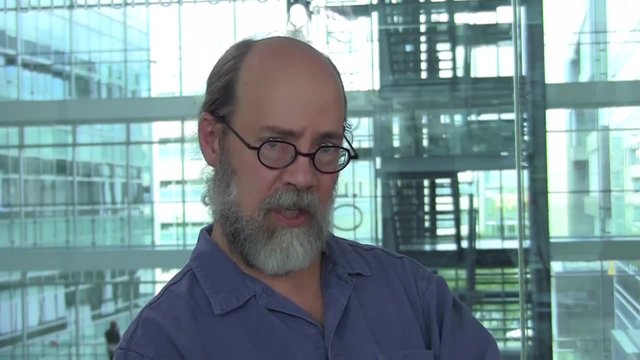 called eyes at the new jersey institute of technology. there was a system called planet uh by folks at the institute for the future in palo alto. there was something in michigan. so so back in uh late seventies, uh early eighties, there were. 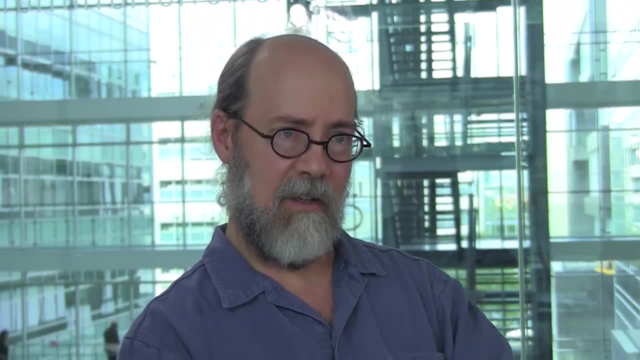 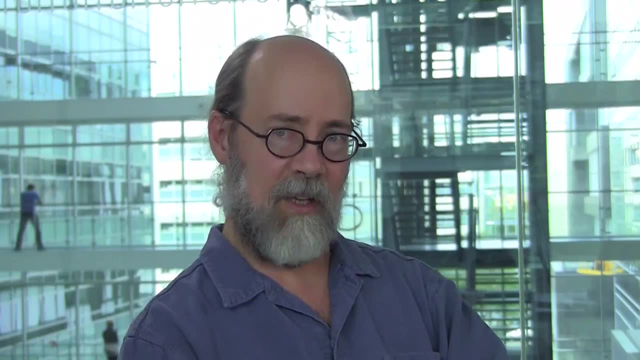 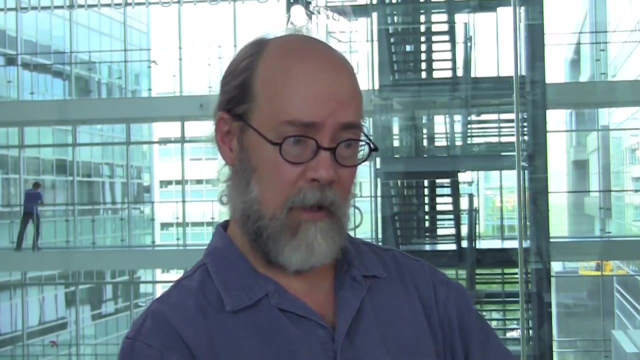 a lot of online communities uh emerging and uh, certainly that's where you can see the beginning of of what i'd call social computing research. you have lots of people, they're interacting and you're trying to understand what on earth is going on and you start to see the beginnings of 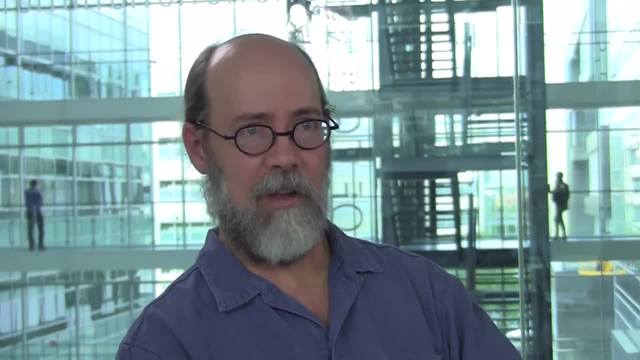 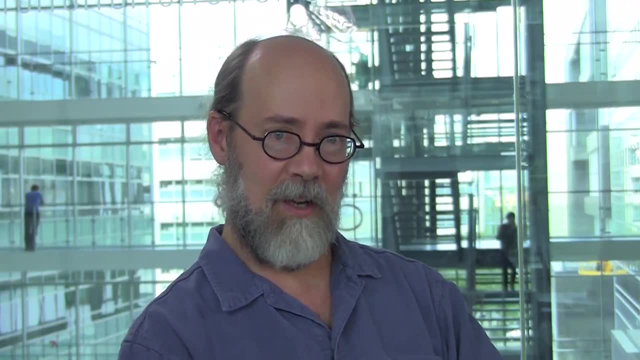 of people self-organizing and you start to see the beginnings of of people self organizing, or people uh uh, or self organizations fragmenting. so you have the emergence of flaming right and uh uh. you know various types of of cyber vandalism where people are.